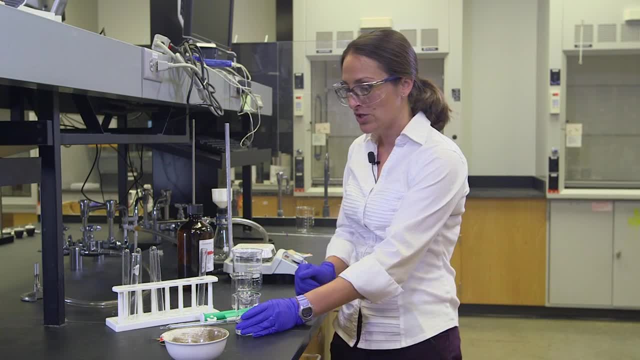 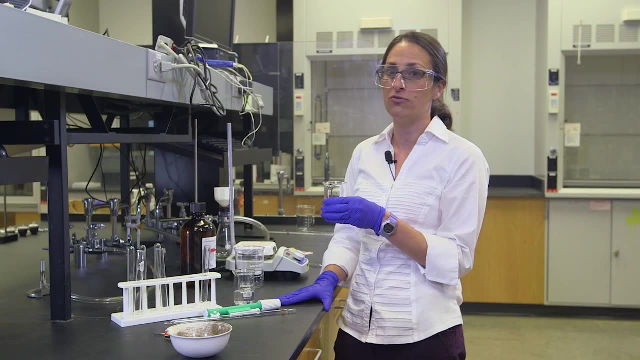 we're going to record is the smell. So, as chemists, we have a special way of determining the smell. We don't want to stick our face in the beaker, especially if it's something like sulfuric acid that can do some damage. So what we do is called wafting, And so we'll. 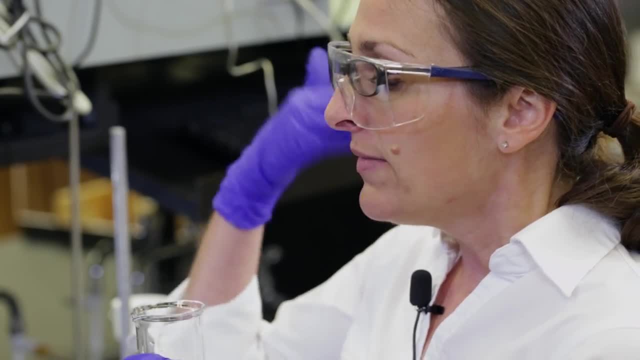 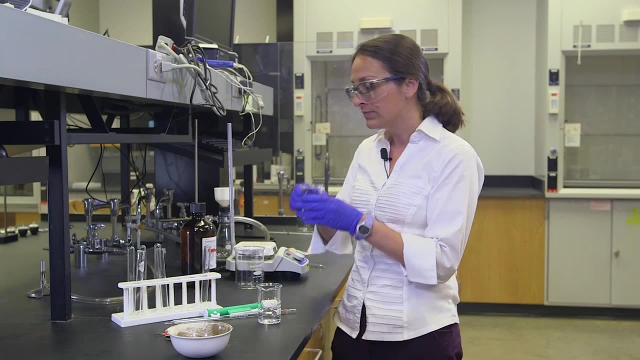 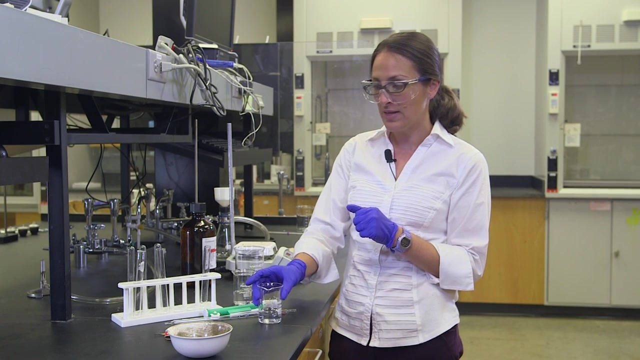 hold the beaker in front of our face and sniff as we're waving the fumes towards the nose. Now, this one I can smell right away. This one smells like nail polish, so I know that's acetone. This one doesn't smell like anything, so I can't determine based on the. 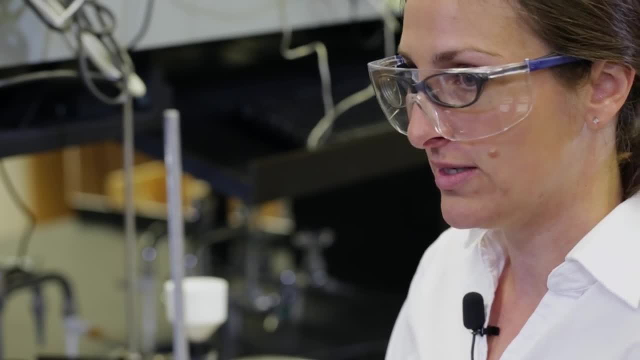 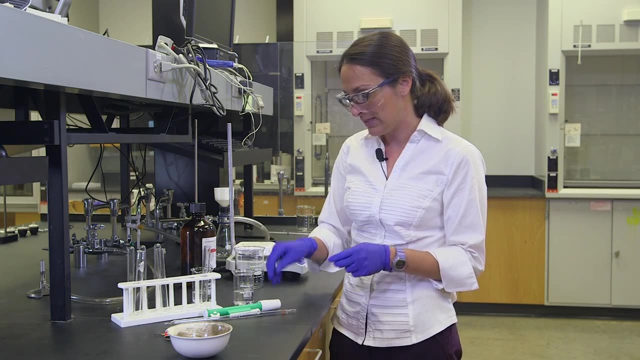 smell what it is. So that's one of the things that we're going to ascertain in this experiment- is: what is the smell? Another thing we're going to do is the flammability test. Okay, so I'm going to take my pipette. 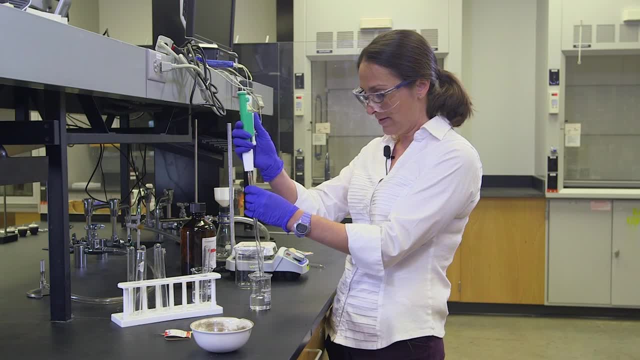 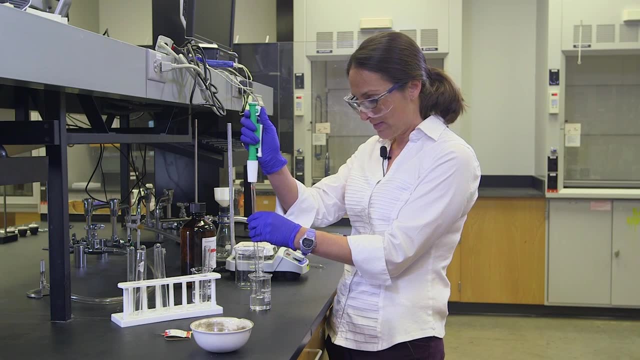 I'm going to treat every liquid as though it's flammable and I want to take less than half a ml. This is a graduated pipette so that I can tell the volume, And there's a dial at the top. I want to make sure my tip is immersed in the liquid before I scroll. 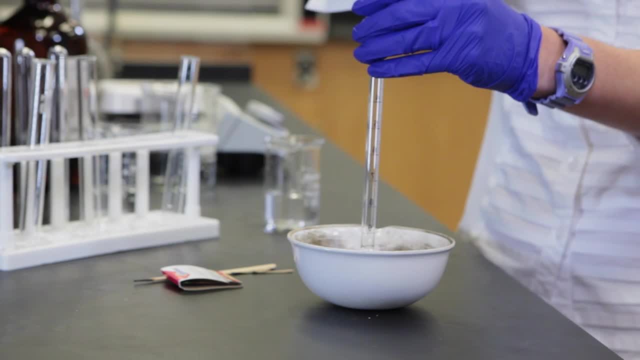 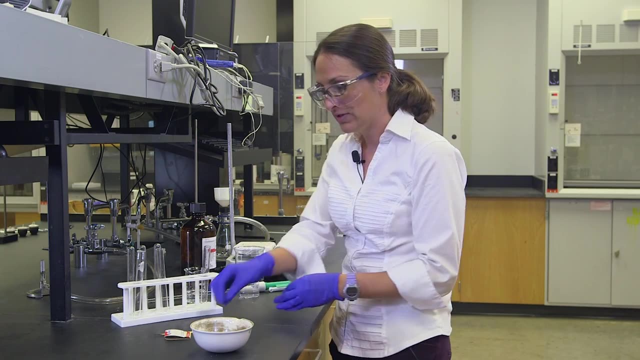 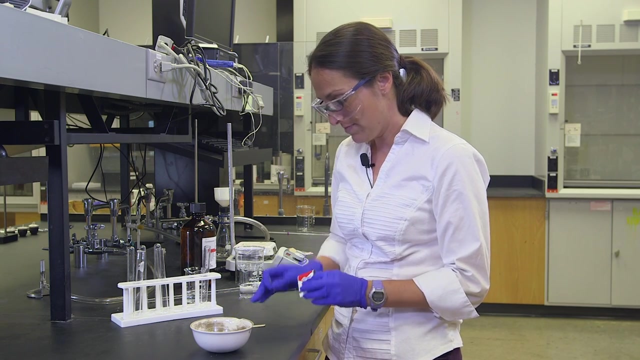 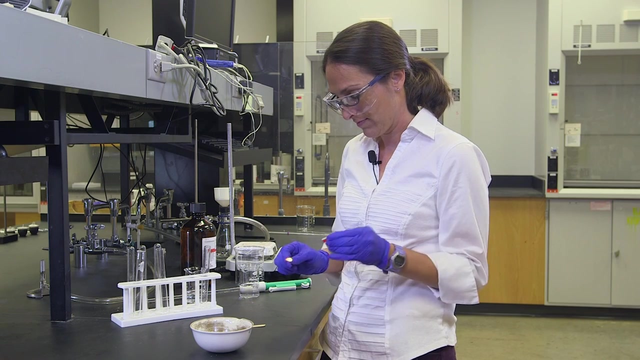 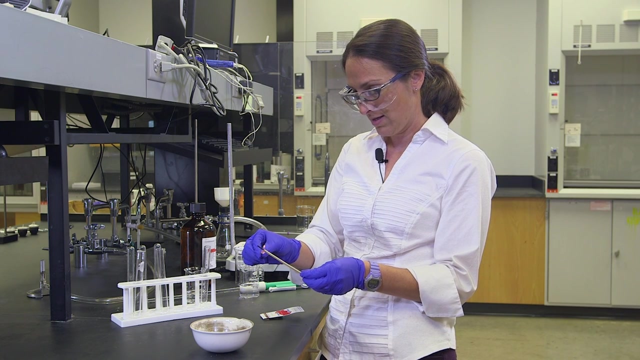 the dial I'm going to transfer, that I'm going to move these larger amounts of liquid away because, again, I want to treat them all as though they are flammable. I'm going to light my splint here. It's a good reason to have your hair tied back whenever. 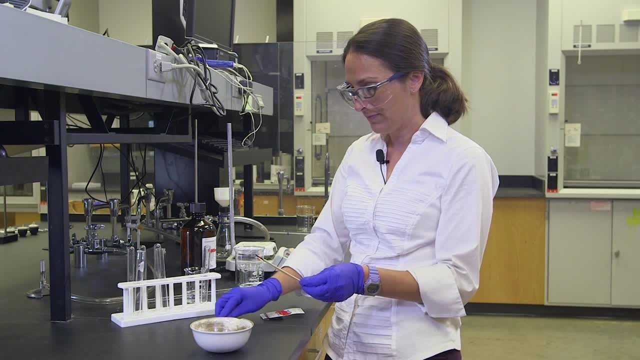 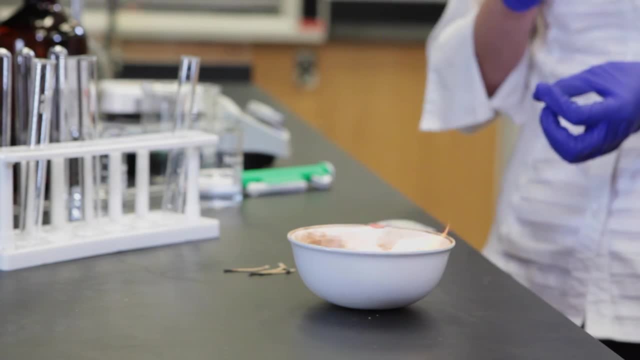 you're dealing with open flame, And then I'm really carefully going to lower this down. If it's flammable, even the fumes will catch fire, And it is. I've taken away the source of the flame and it's still burning. So this is an example. 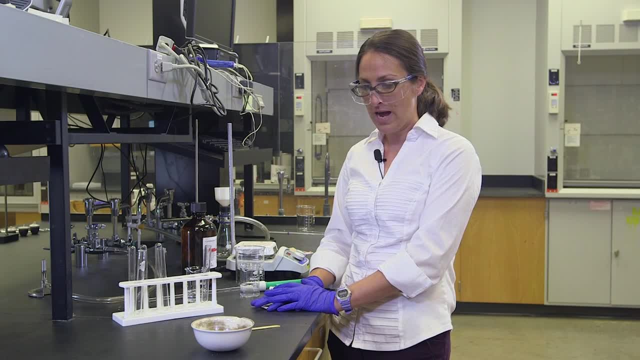 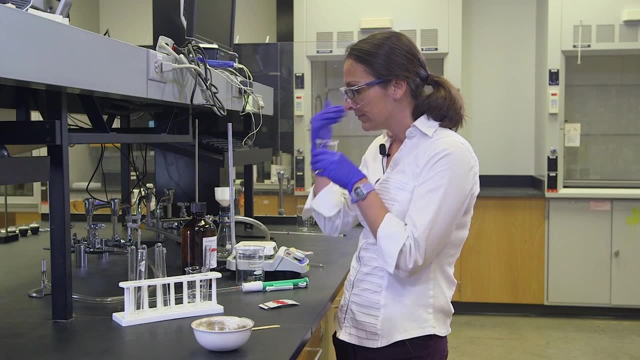 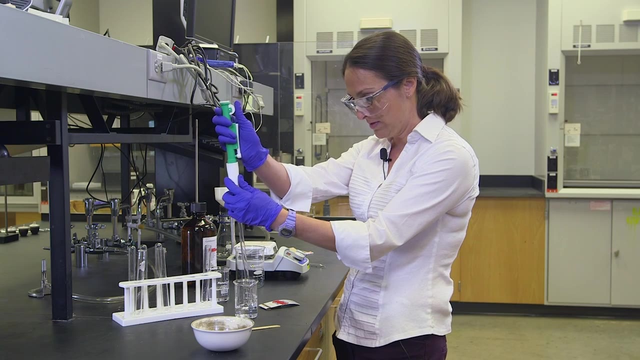 of a flammable liquid. Again, I want to keep my match pack away So I can test another liquid for flammability. Again, I'm going to treat all of these as though they are flammable, So I want to take less than half a ml If I have too much volume. 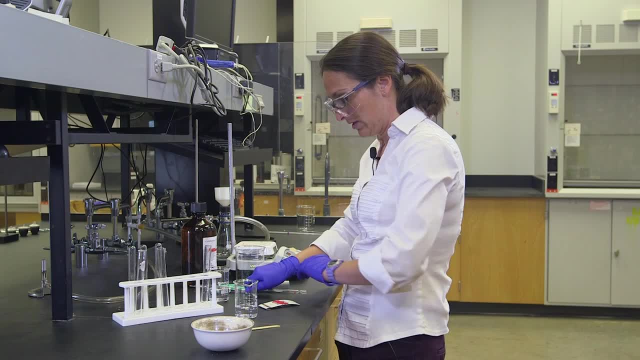 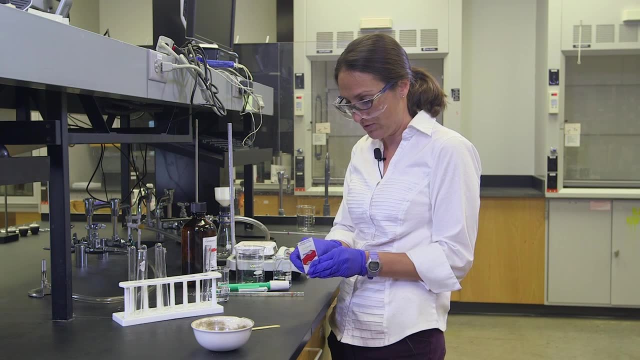 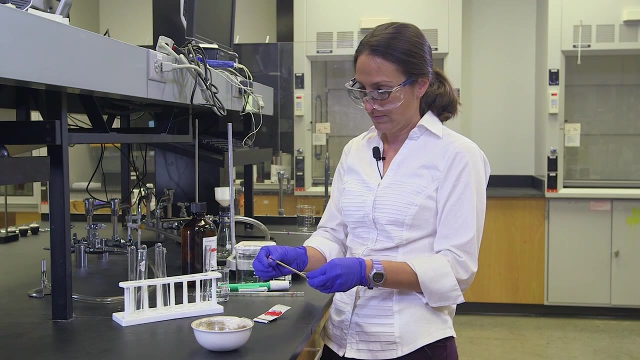 what can happen is I'll get a really big flame, And that's too dangerous. I'm going to move my larger source of liquid away because, again, I'm going to treat them like they are all flammable. I'm going to light my splint again. 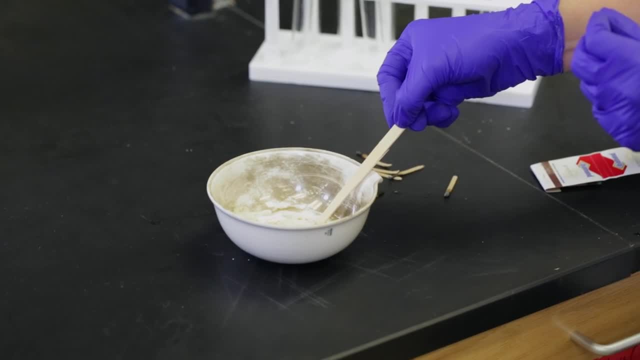 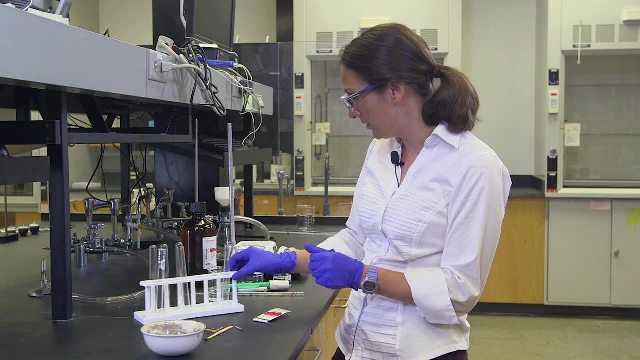 I'm going to lower it into my bowl. In fact, this put the fire out, so this second liquid that I used is not flammable. Subtitles by the Amaraorg community. One of the other things that we'll determine is miscibility, and this is really like a. 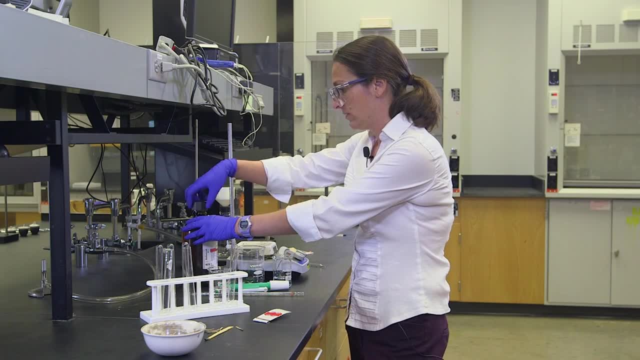 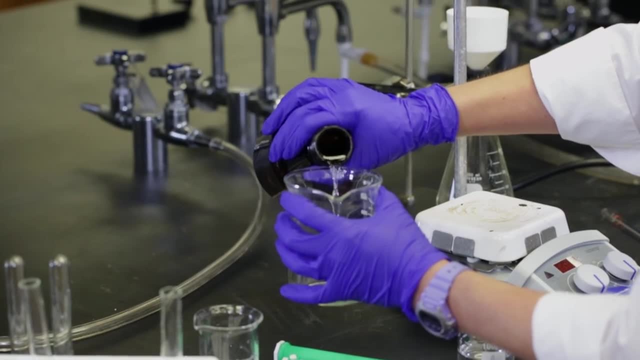 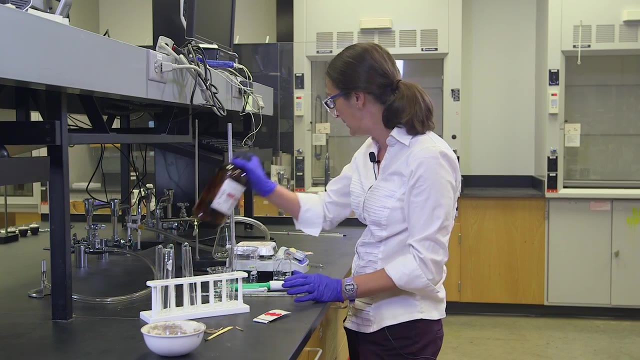 solubility for liquids In our lab. we're not going to have you use your pipettes to remove your reagents. We're just going to pour a small amount into a beaker and then we'll transfer from that beaker. This prevents contamination of our reagent bottles. 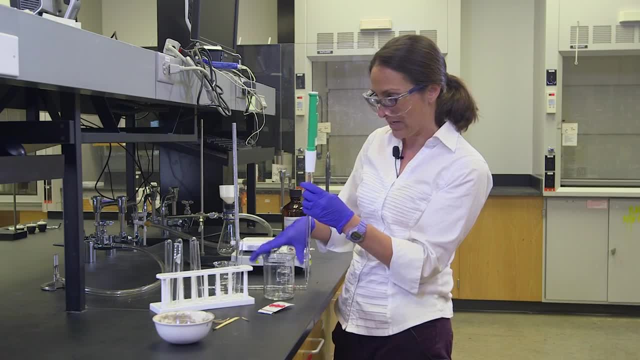 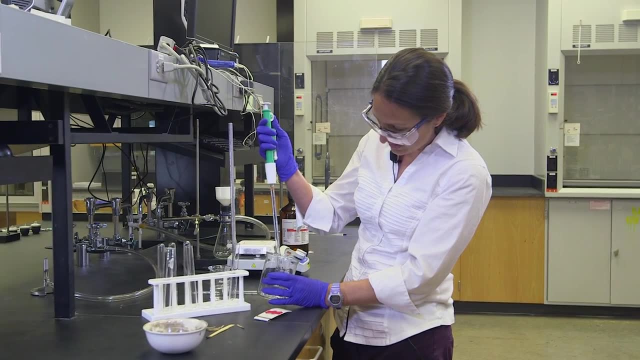 Subtitles by the Amaraorg community. I'm not really concerned about measuring it, I'm just going to add enough that I can see some aliquot into the test tube. You can use the pipette for this, or you can just pour it in. 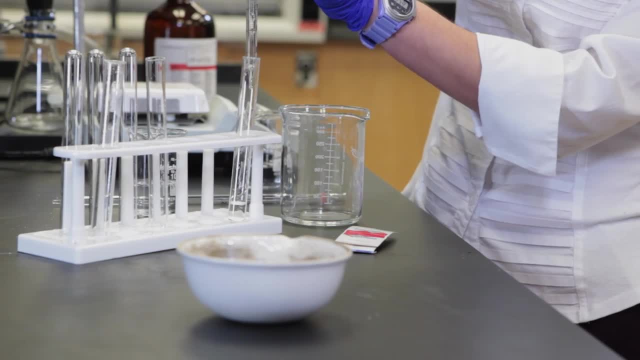 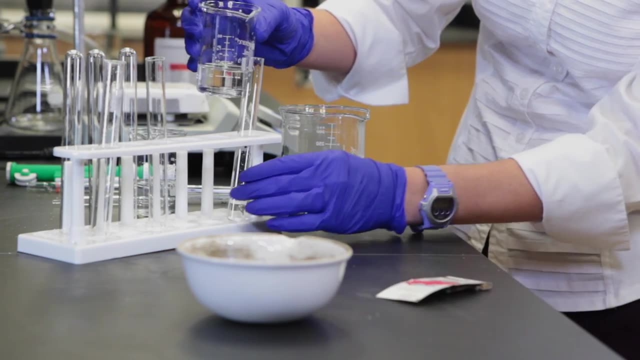 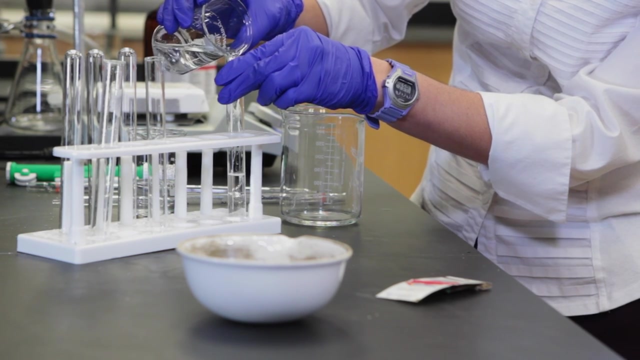 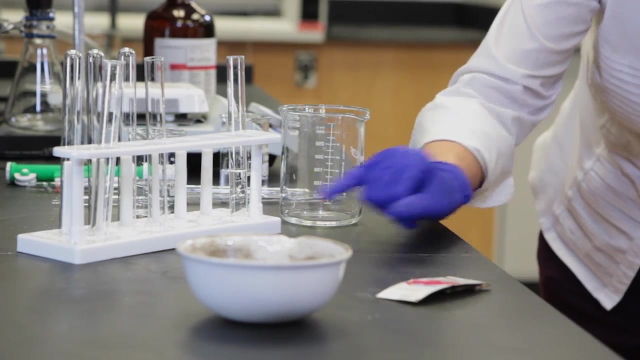 I'm going to add my second liquid. What I'm looking for here is whether they mix completely or whether I see two distinct layers. I'm going to pour it in slowly. Subtitles by the Amaraorg community. All right, so this is an example of immiscible liquids, liquids that do not mix together. 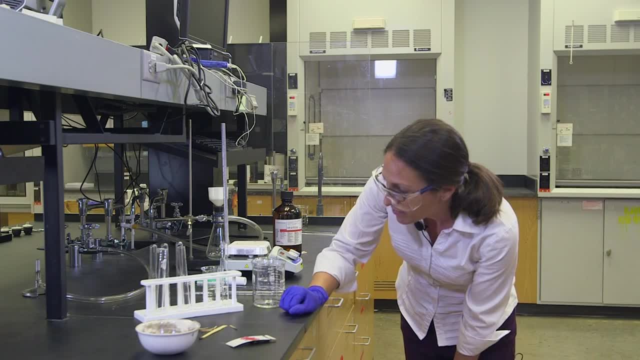 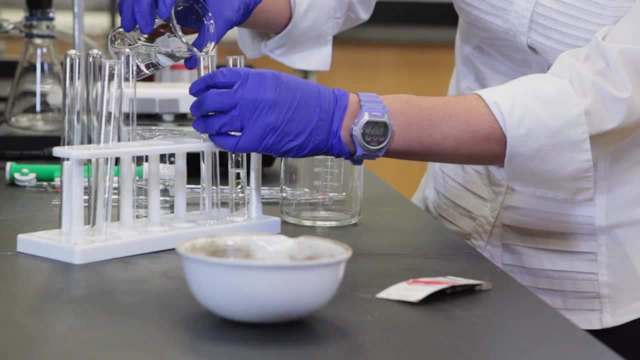 completely. I can tell that because there's a distinct layer separating the two liquids. Let's try another example. Again, I'm not really concerned with measuring here, I just want to combine enough to see Subtitles by the Amaraorg community. 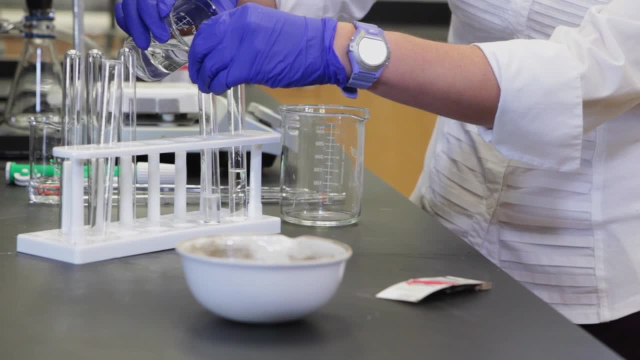 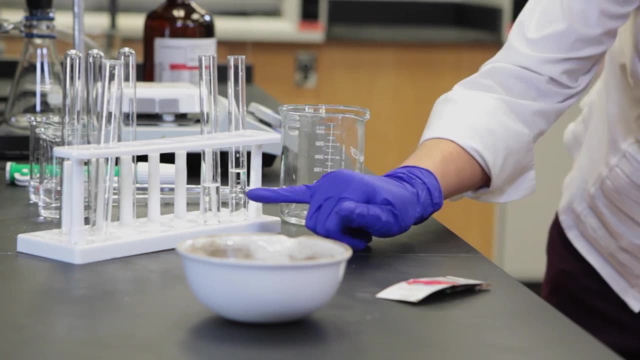 So now I'm going to mix different samples- Subtitles by the Amaraorg community- And again I want to see if they mix completely, if they are miscible or if I see a distinct layer. This is an example of miscible liquids, because I don't see any distinct layer And you can.